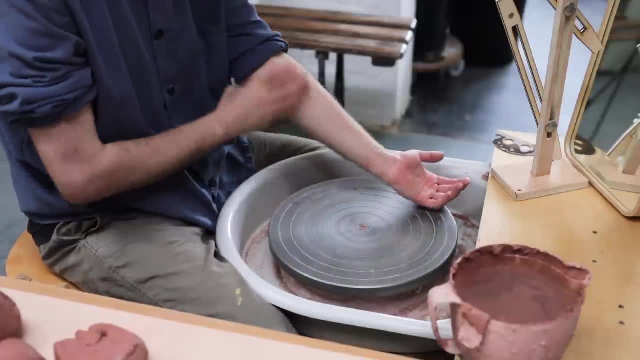 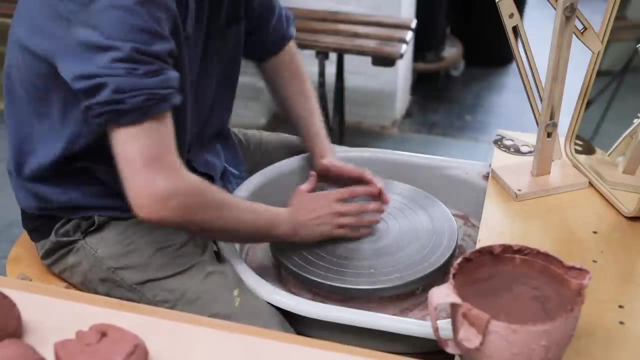 I then take my left arm and I shove my elbow into my torso And I lean my upper body weight forward slightly onto that arm to stabilise it. What you don't want is both of your elbows up in the air like this as you're trying to centre, as they aren't braced against anything. 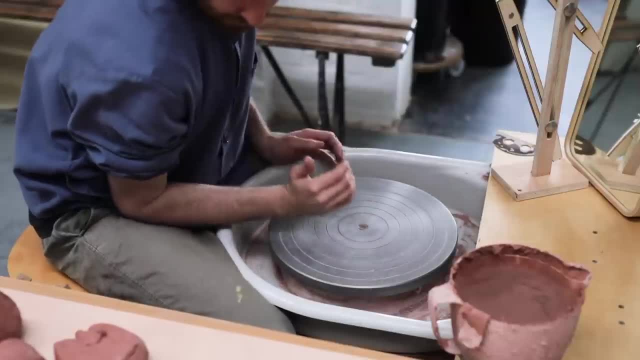 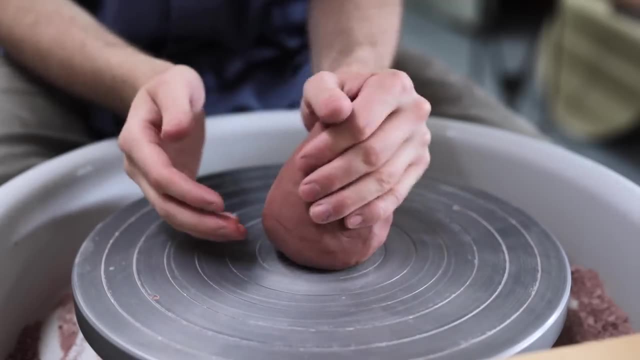 So instead, I tuck my elbows into my waist and I lean my upper body weight forwards onto them. The first thing we need to discuss, though, is attaching the clay down to the wheel head, Like we spoke about earlier. it helps to have an even round shape that's thrown against the wheel. 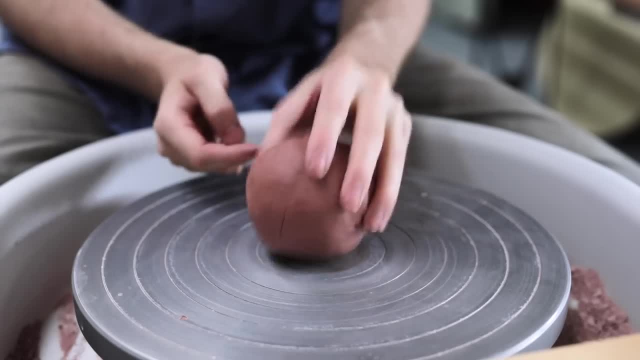 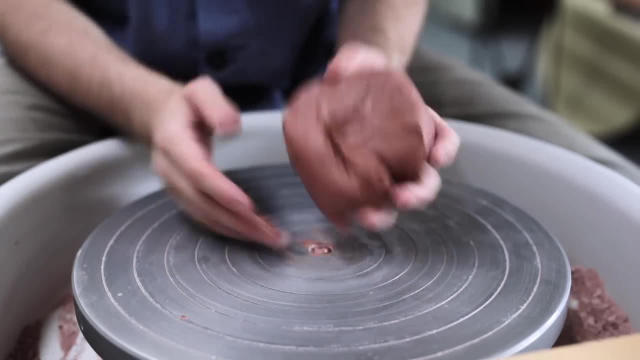 This way, no air can be trapped beneath the clay when it's slammed down, And you can see just by placing it roughly in the middle how centred it was. Compare that to this irregular lump which, even when placed in the centre, spins and wobbles on its central axis. 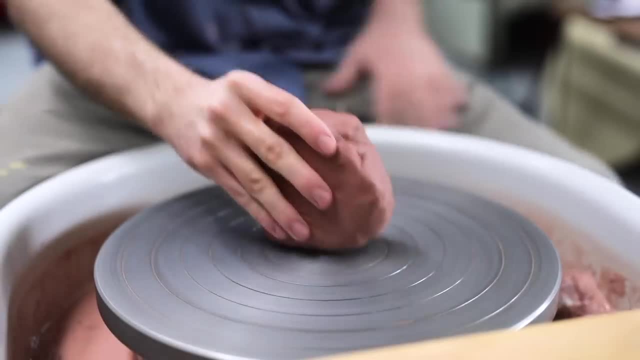 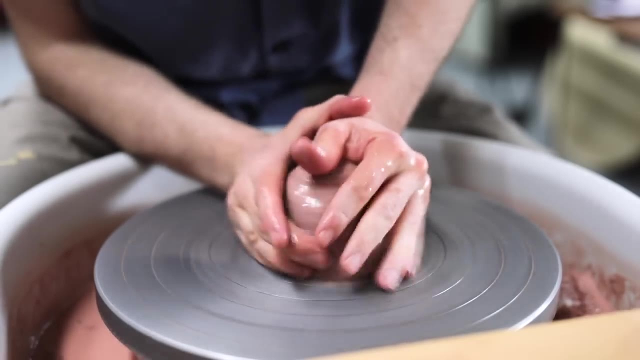 And you'll see, when I try to centre a piece like this, how difficult it can be to centre as those undulations slap into your hand as the lump spins around, And for a beginner this can be quite difficult to control. So don't use lumps of clay like this. 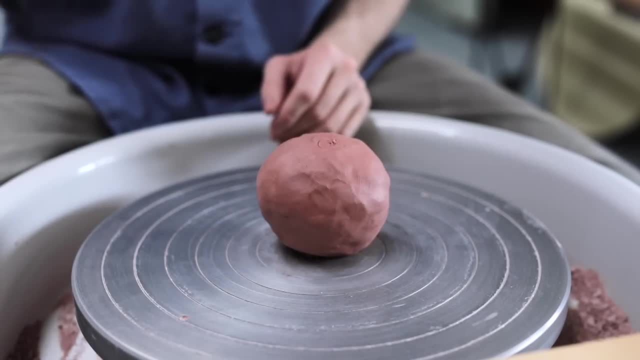 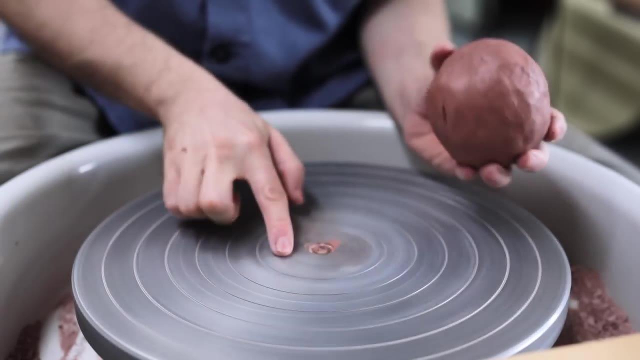 And instead patch your balls of clay into spheres like so, Or at least in the middle, Or into a shape with a rounded base and a conical top. Now the obvious first step is to throw the clay as accurately into the middle as you possibly can. 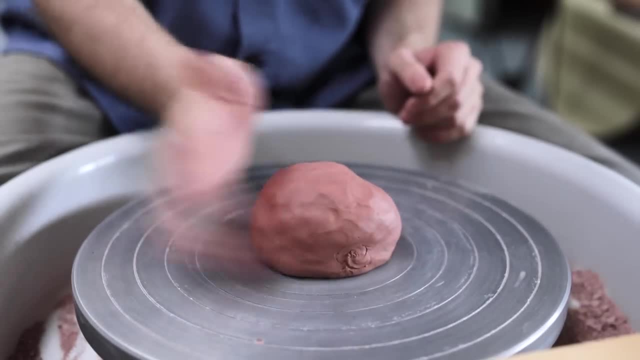 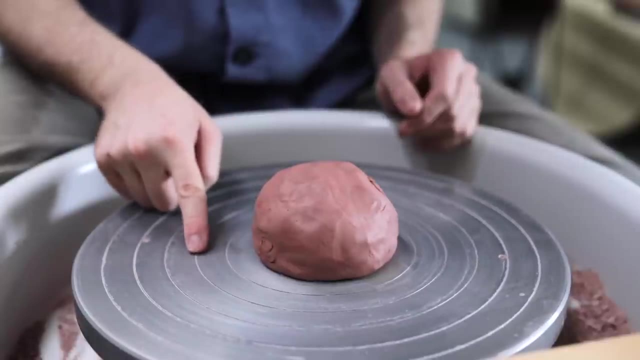 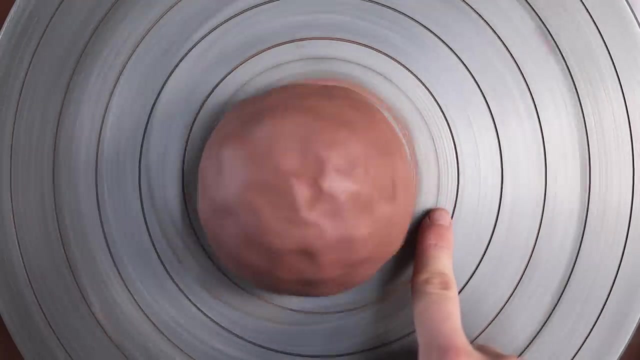 And to slam it down firmly. This way, it sticks onto the metal, And one thing I do is use the rings that most wheel heads have in order to tell if the lump of clay is in the middle, Because as you spin the wheel, you'll notice that the lump of clay will probably have a larger gap on one side as compared to the other. 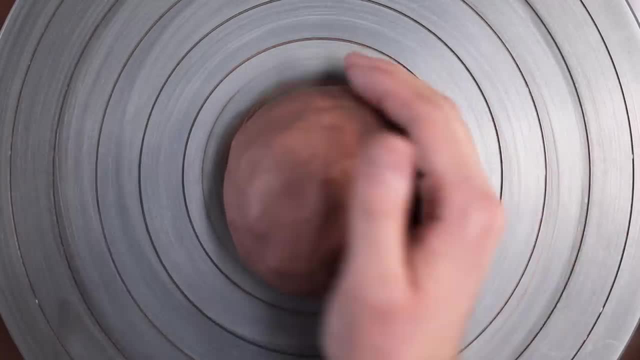 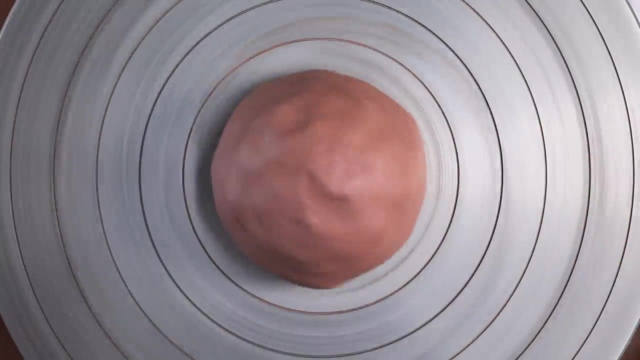 And all you need to do to remedy this is to push the clay away from where it's closest to the line Until the gap between the clay and the line is more or less the same all the way around. At this point you can even pat the lump of clay into shape a bit. 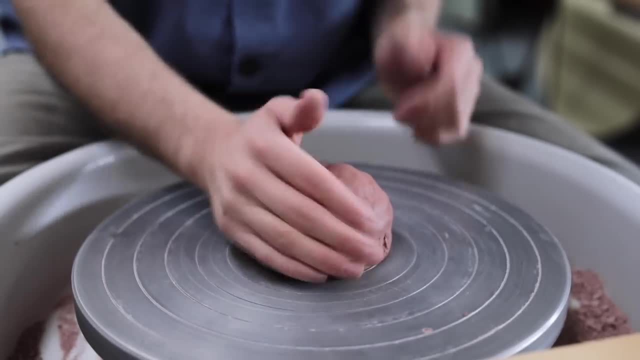 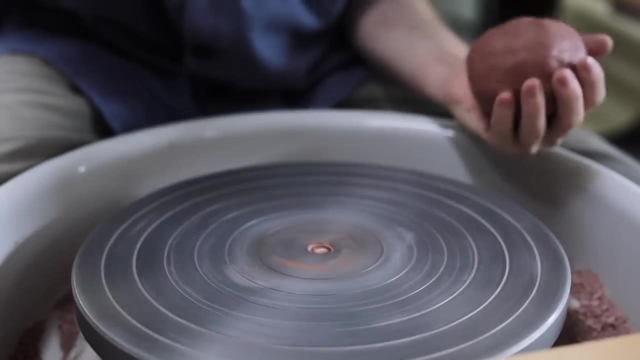 To get it as centred as possible before you begin to add water to it and begin the process properly. Initially attaching it very firmly is crucial, though, And what you don't want to do is slam it down onto a surface that's already quite wet. 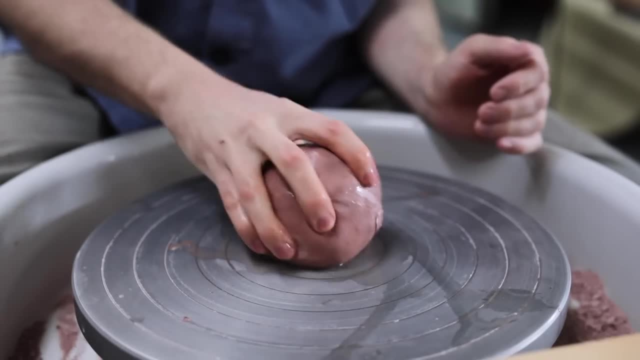 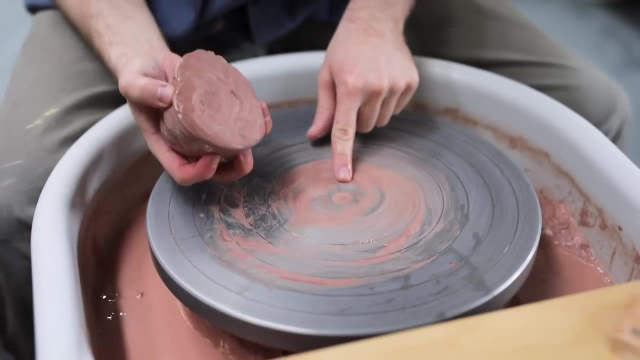 As the lump of clay just won't stick to it properly. So ideally you want a dry wheel head and a dry lump of clay. Otherwise, this is what happens when you begin to centre: The lump will just fling itself off. But there is a remedy to this. 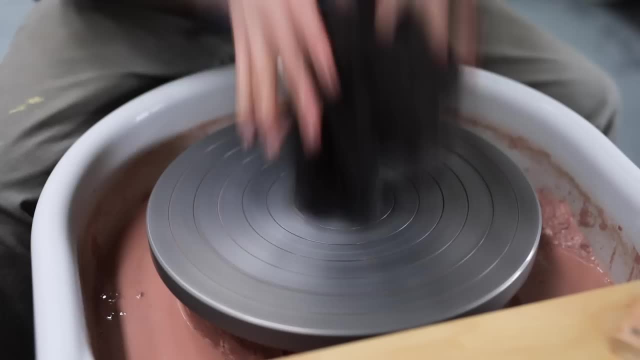 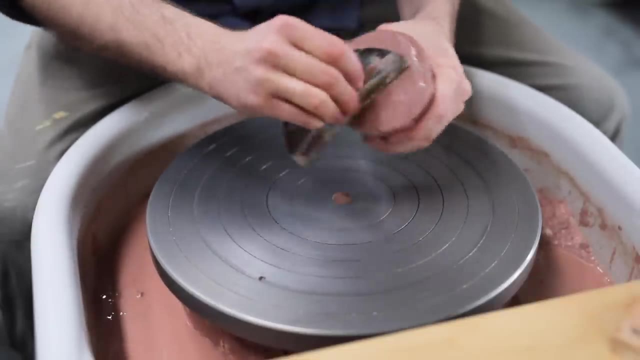 The first step is to clean the wheel head. I sponge away the excess clay And then I dry the metal off with a towel And then take the lump of clay and I scrape away all the wet slip on the bottom of it And then I slam this drier, tackier area onto the metal. 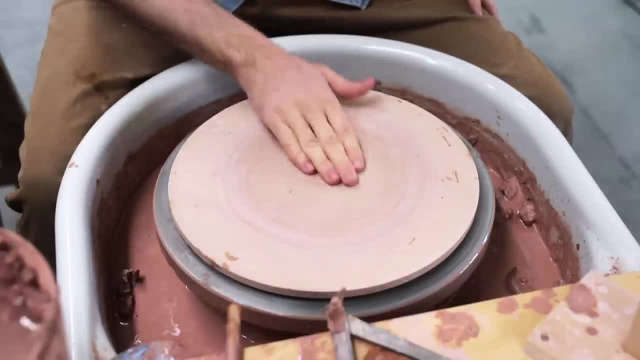 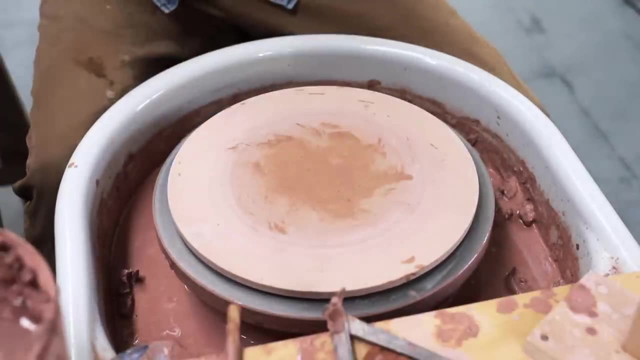 There is an exception To this rule, And that's when you're throwing on a slightly porous surface. In this instance, Such as when I'm throwing on MDF wood, It helps the piece of clay stick if I dampen the surface. 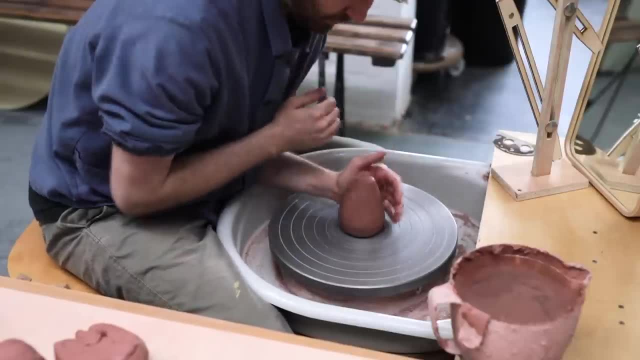 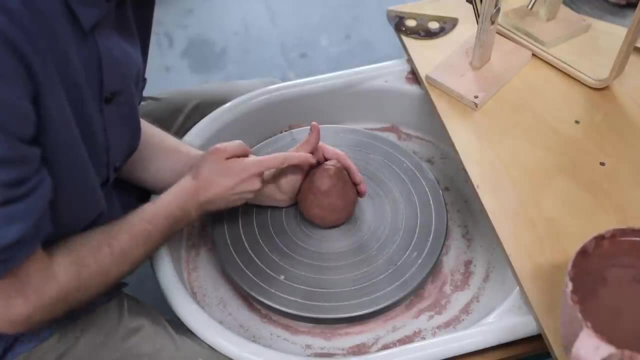 So, to begin, I tuck my arm into my waist And I'm also resting my forearm onto the plastic wheel tray. I then position my forearm so it lines up perfectly with the lump of clay, And I want the ball of my thumb and the base of my palm to be pushing. 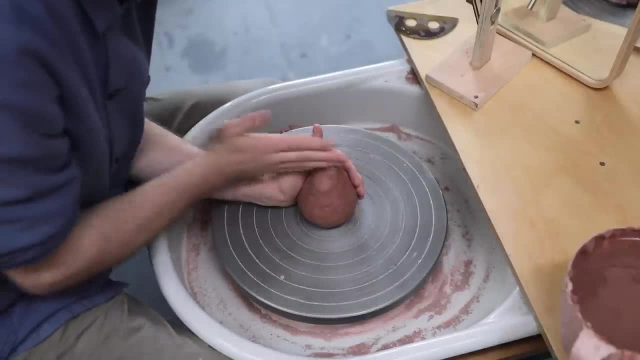 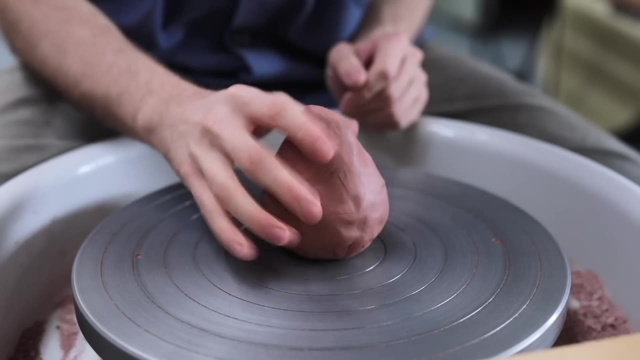 And it intersects the middle of the lump of clay. It's not off to the left like this, Nor is it too far to the right. Instead, you want it, so everything lines up. So now, after all of that, Let's really get started. 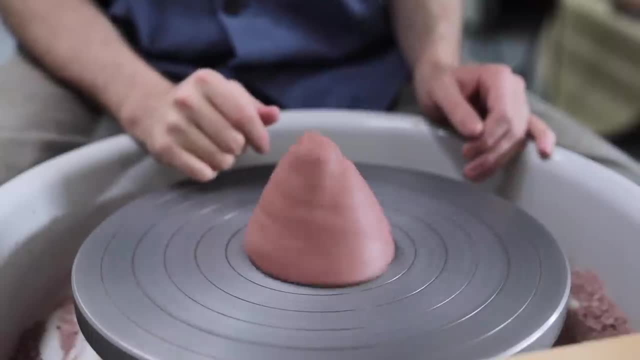 I slam the clay firmly onto the metal wheel head And push it roughly into centre, And you can already see that the piece is quite centred, Although there's a lot more that needs to be done Before it can be thrown into a pot. 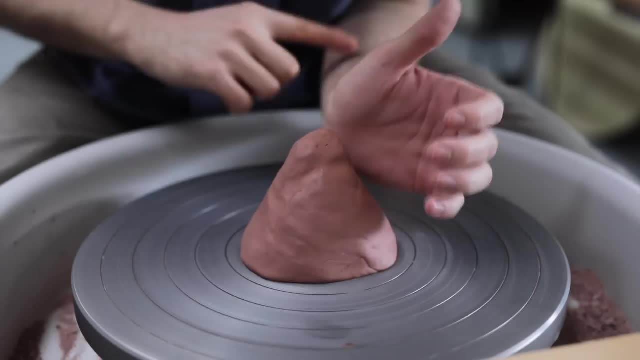 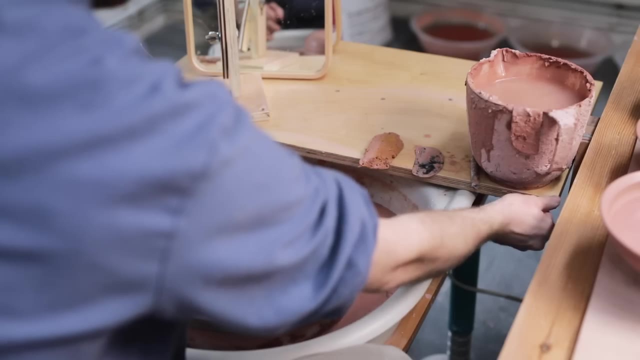 So I begin by bracing my left arm into my torso And onto the wheel tray And I lean my upper body weight onto that arm And I lean all of that onto the lump of clay And I'll use this moment to talk about the importance of water throughout this process. 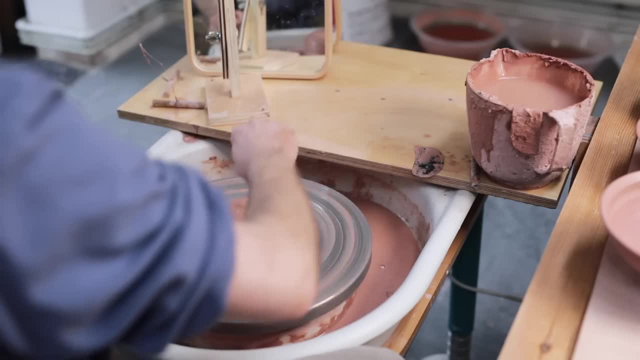 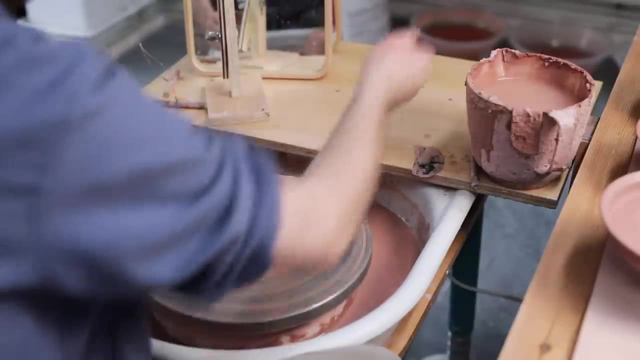 The clay needs to remain lubricated The entire time, Be it with slip or water, And if you ever feel your hands beginning to stick to the lump of clay, Or if you feel any friction, It's time to add more water, Which I typically do just with a cupped hand. 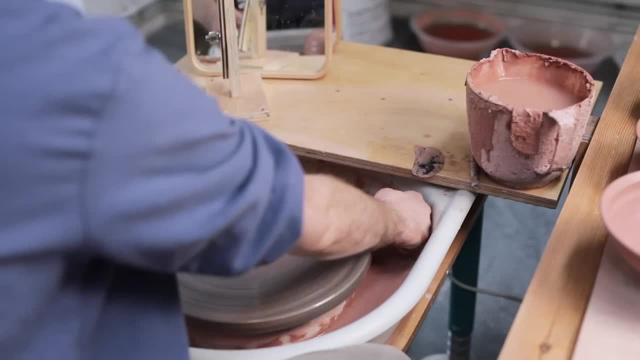 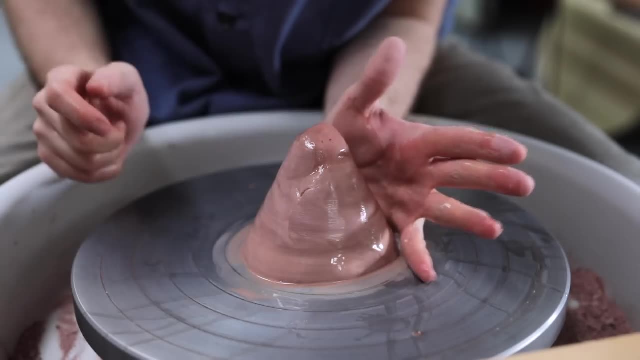 Or I sometimes just keep a sponge handy Which I can dip into the water in the wheel tray To soak it up And squeeze it out onto the clay As my left hand's palm pushes in, I take the little finger of that hand. 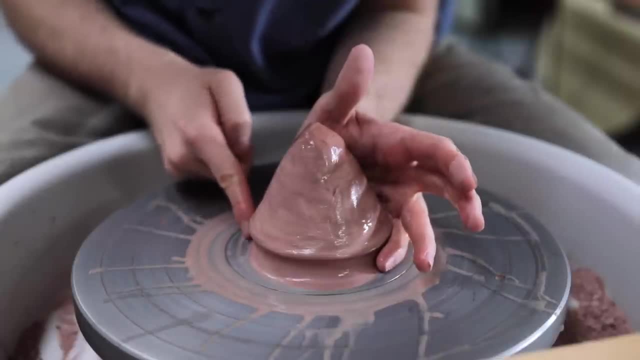 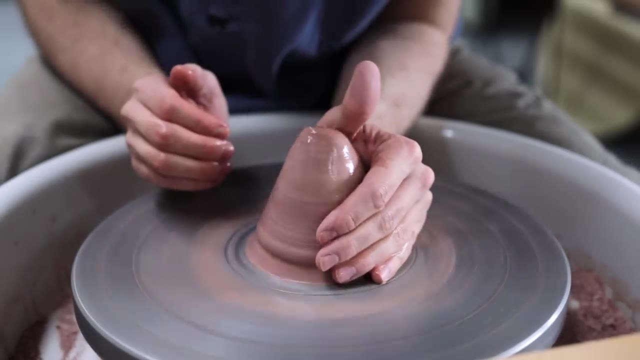 And I squeeze it around the base Firmly. This creates a seal against the metal wheel head And another barrier to ensure that it's stuck down securely. It also neatens the clay around the base And simply stops it from spreading out onto the metal wheel head. 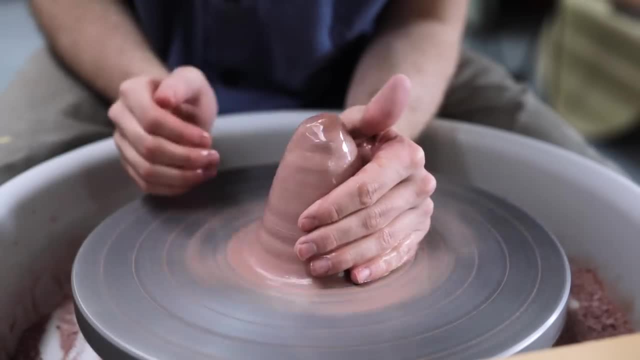 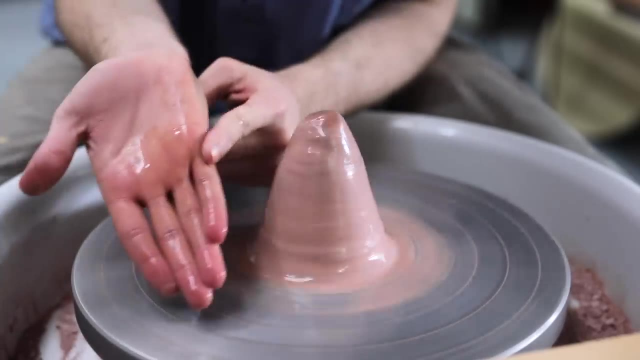 So far I've only been applying horizontal pressure To the piece of clay, Which means the lump will become ever more conical. So I need to introduce another hand Which applies some vertical pressure, With my right hand To push down on the piece of clay. 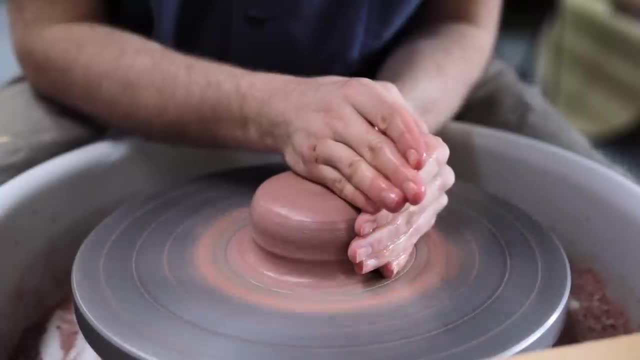 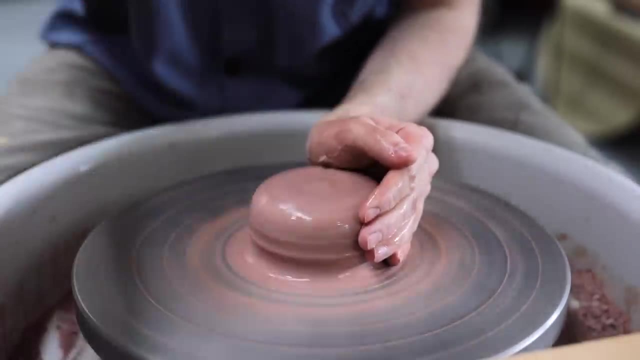 To contain it. I push down directly over the middle of the piece of clay, Matching the pressure my left arm is applying, And I corral the piece of clay into a disc shape, Like so- And this part is really important- Applying both an even pressure from the side. 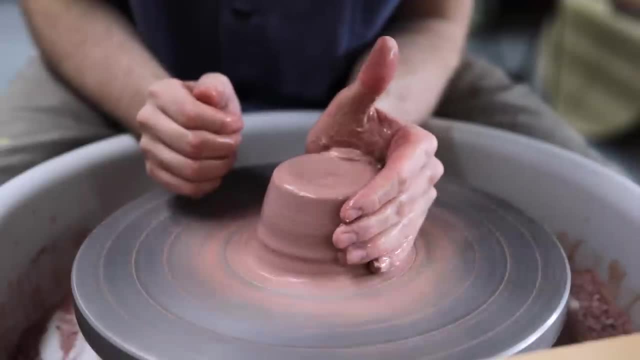 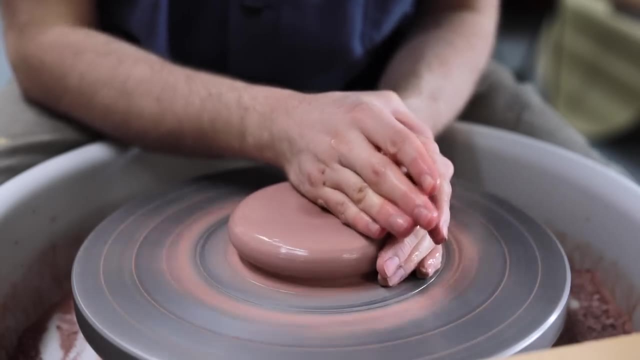 And the top, As if the pressure exerted with my left hand is too great, The lump of clay will cone up, And if I push down too firmly with my right hand, I'll squash the piece of clay down Into a pancake. 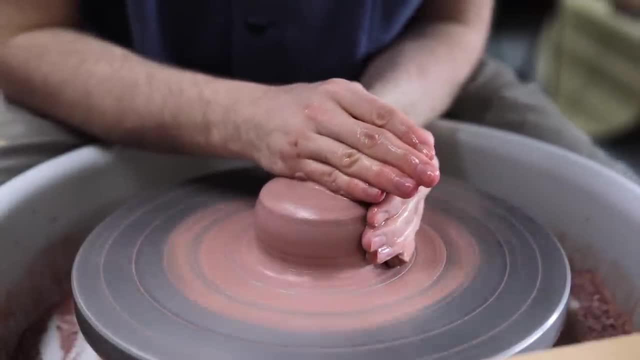 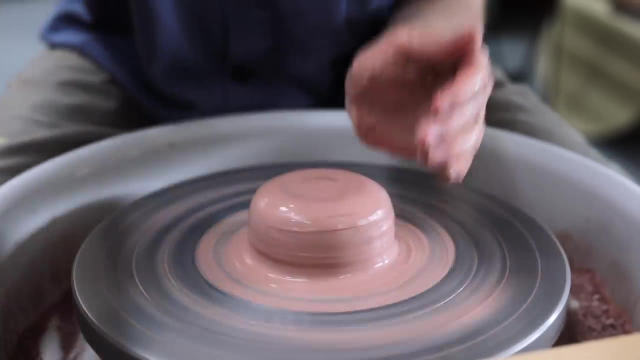 That's an even amount of pressure From both the side and the top, Which is what we're after, And I sometimes take the slip from the wheel head itself, Like so, To lubricate the lump. Those are the hand positions I use. 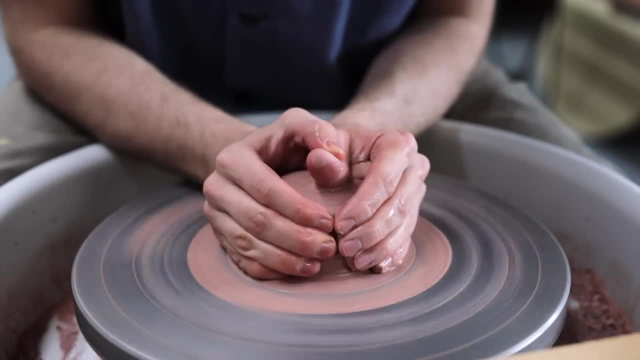 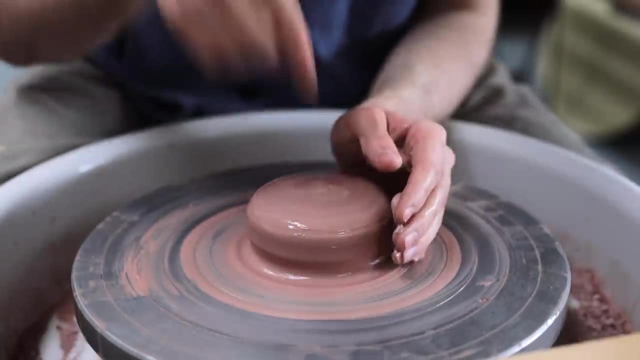 But there are others. For instance, you can apply pressure from both sides And then use your thumbs to apply downward pressure. But personally I find this a little bit uncomfortable And I feel as if I have a lot more downward control When I use the side of my right hand. 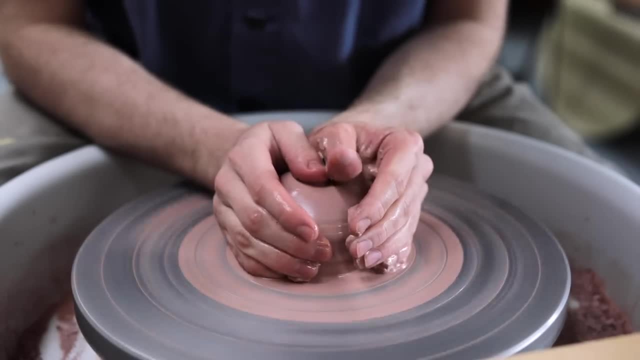 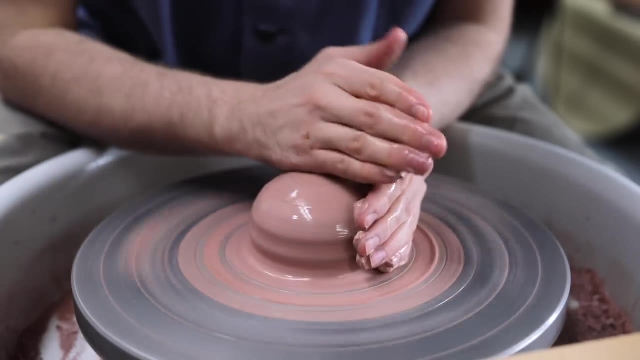 In order to push down, And as I centre The lump of clay with all of my digits Of my left hand, As if I'm gripping a ball tightly, And as all those fingers are squeezing And I'm leaning in with my left arm. 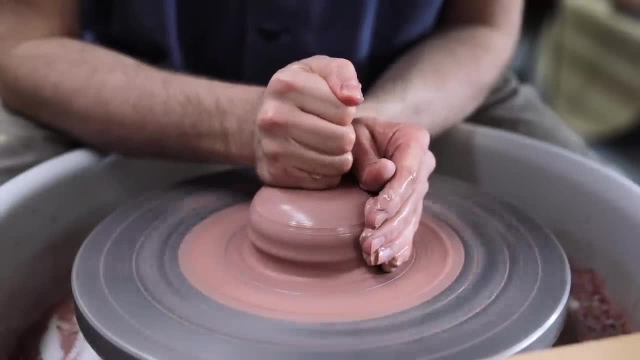 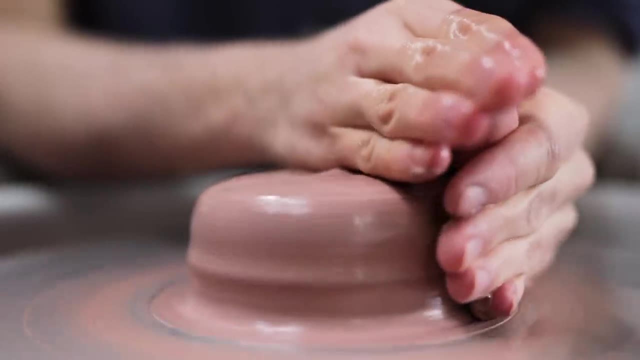 My right hand pushes down from on top. It's worth knowing that probably every potter out there Centres a little bit differently. We all follow a similar set of rules But ultimately our hands are all different sizes And shapes And that affects how we hold them and use them. 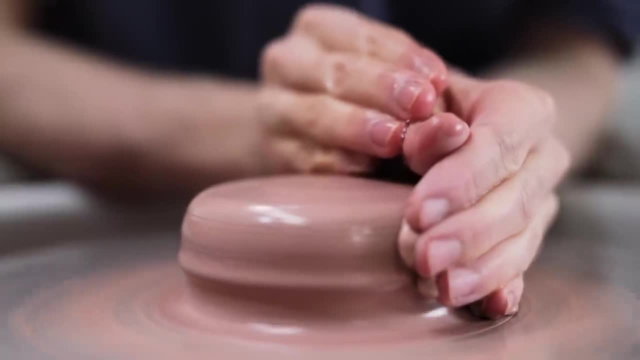 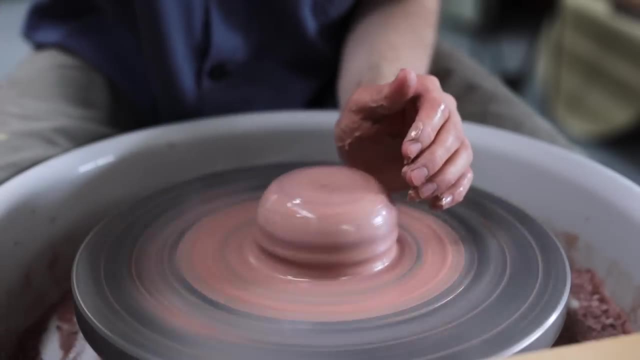 For this process, So don't be surprised when you see potters doing this process. They're still essentially following the same principles, Just in slightly different positions. One thing that's important Is to not let the clay control your movements, For instance. 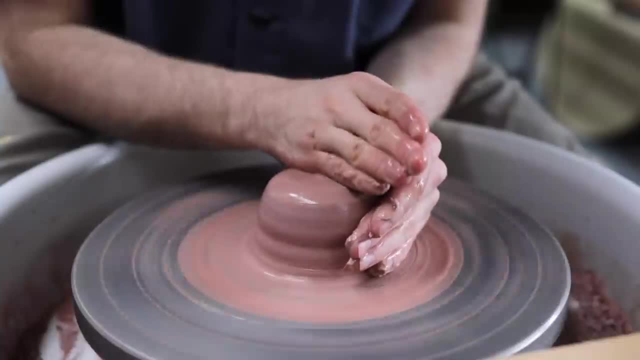 I place my forearm down so securely That the clay has to conform to the shape I've given it. If the clay is wobbling, You don't want to let your hand simply follow the wobbling piece of clay. Instead, you need to position your arm. 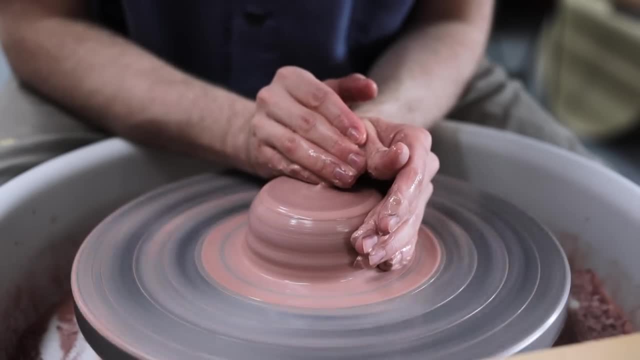 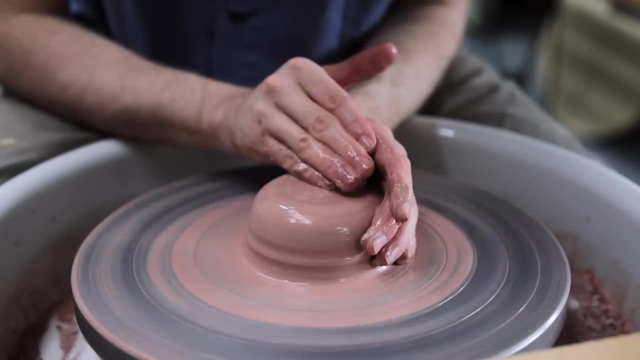 And your hand so securely That the soft, wet clay Has no other place to go Other than the area you've designated for it And the shape you see here. It's a good starting point. It has a flat top And only very slightly curved sides. 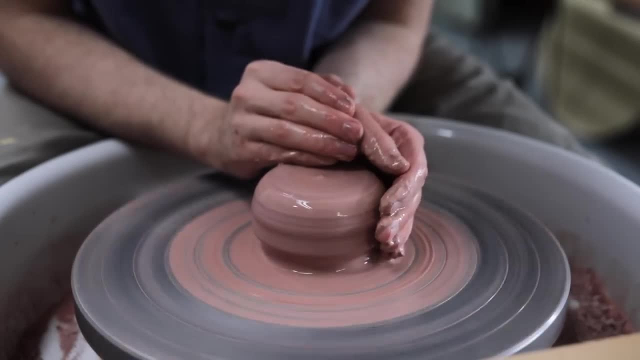 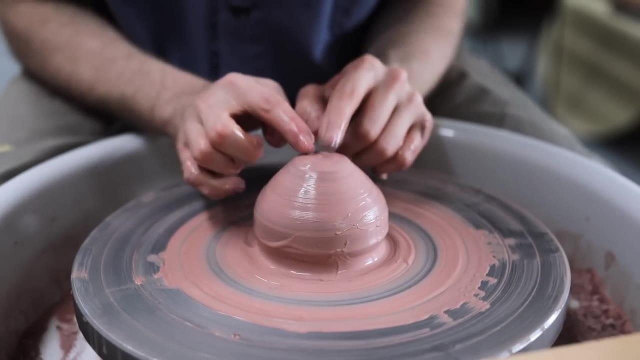 That meet the wheel head flush. You don't want a piece of clay which has too much of an indentation At the bottom, As now the centre of gravity is slightly higher And you might have a harder time opening it up later on. You also don't want a shape that bulges up in the middle unnecessarily so. 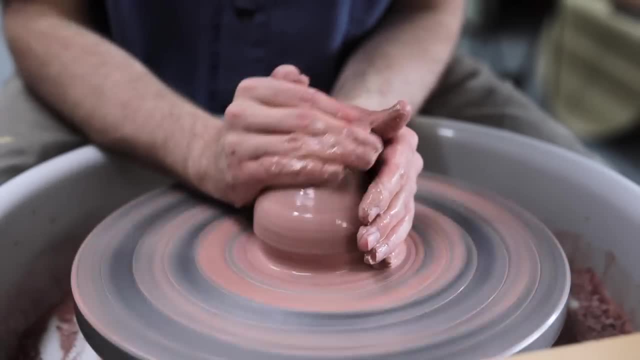 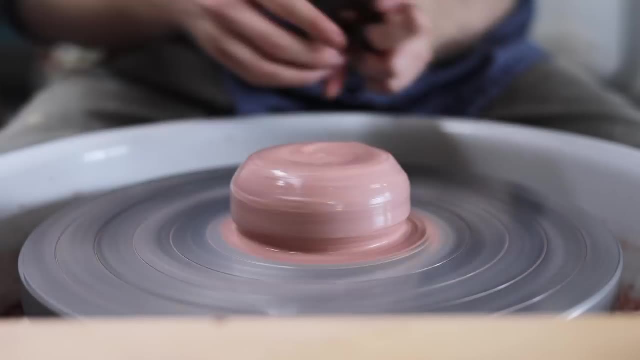 As that means you have to push down further, And perhaps unnecessarily so, When creating the hollow And forming the base of the pot, If you happen to be using a clay which contains quite a lot of grog, One that's quite coarse. 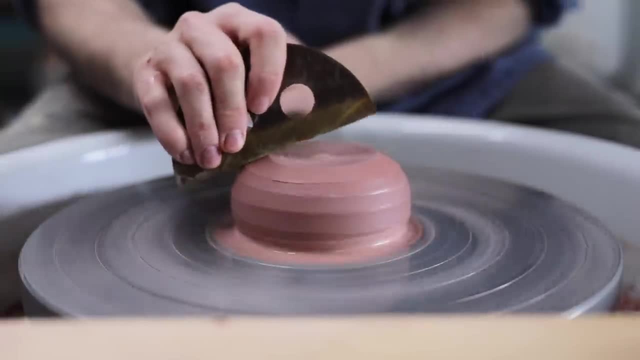 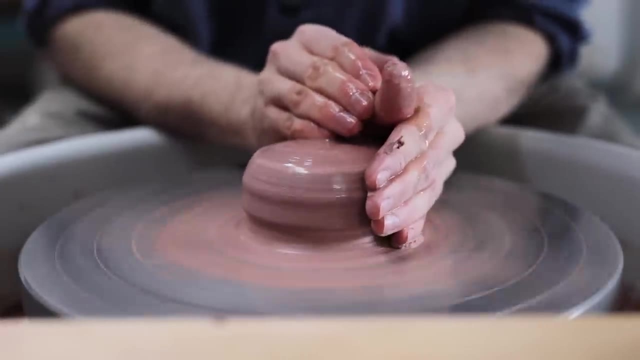 And you feel like the surface is starting to feel like sandpaper, It's best to scrape away the outermost layer And then proceed with centering as normal. It's also worth knowing That if you are feeling this, You're probably taking too much time to centre your clay. 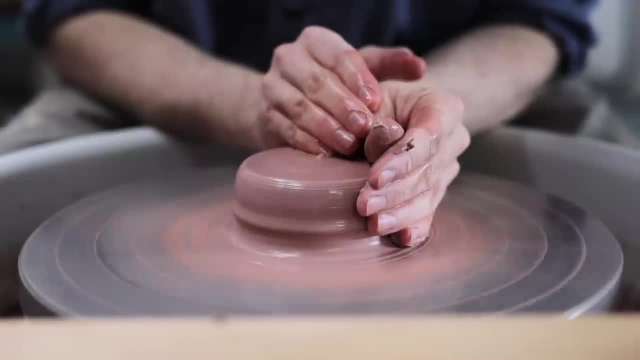 It isn't a process that's worth rushing at the beginning, But you also don't want to spend 10 minutes doing this Every time you make a pot. Otherwise you'll never make anything, And ideally, this is a process that you should be able to complete. 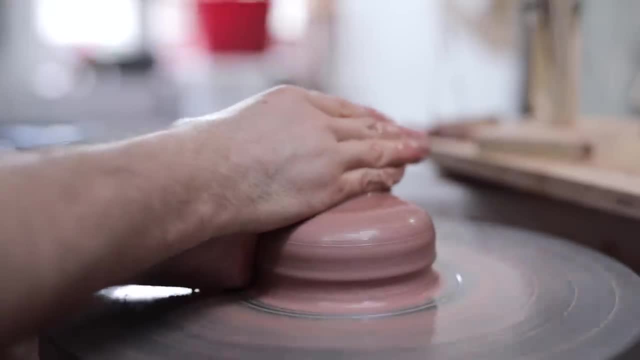 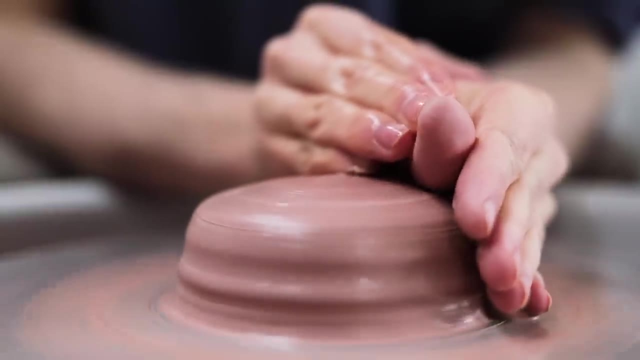 In about 10 to 40 seconds, But this does depend, of course, on the size of clay, And larger lumps can take much longer, But this is a process. Another thing we should discuss Is the speed at which the wheel is spun. 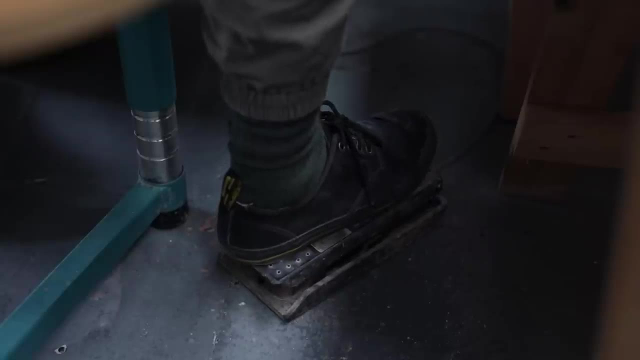 You don't want to do this process really slowly Because once again It'll just mean it takes longer. And say, when you are throwing dozens of bowls and mugs, You really want to minimise the amount of time you spend centering the clay. 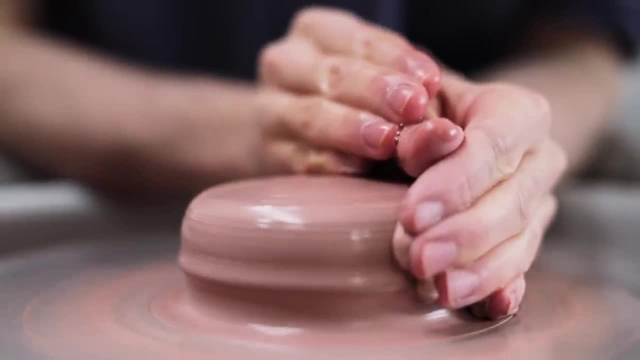 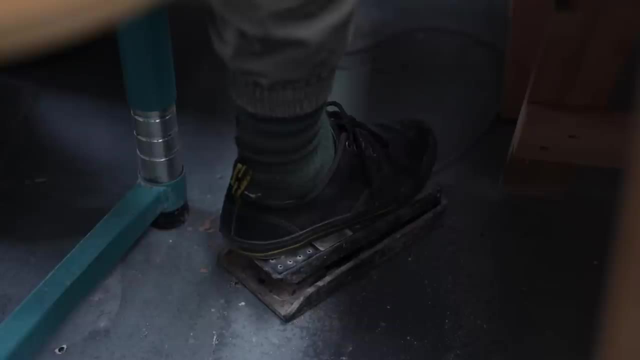 So I spin the wheel very quickly, Although I don't max it out- In fact, I never really do. There's virtually no need to ever put your foot down all the way- But I do spin the wheel quickly, Fast enough That, however, I push my fingers and hands into the lump of clay. 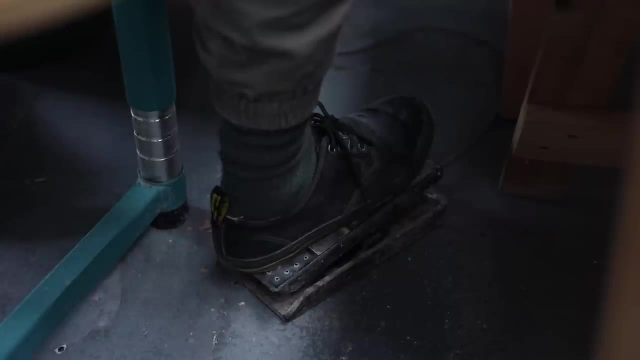 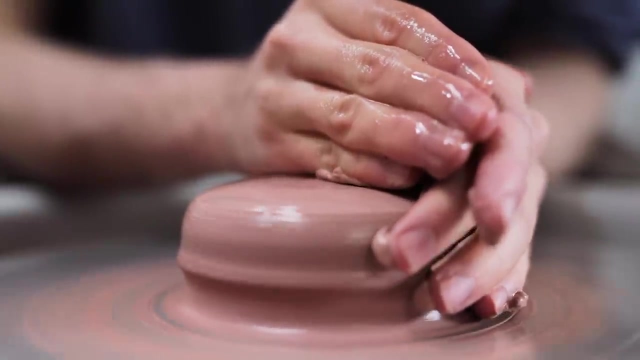 It affects the entire piece Practically instantly, Which means you want it to be rotating many times every second. If you spin the wheel too slowly, It means you need to linger With each movement you place on the lump of clay To ensure that it remains the same. 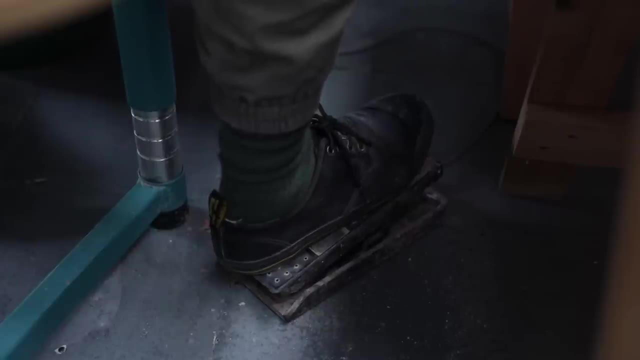 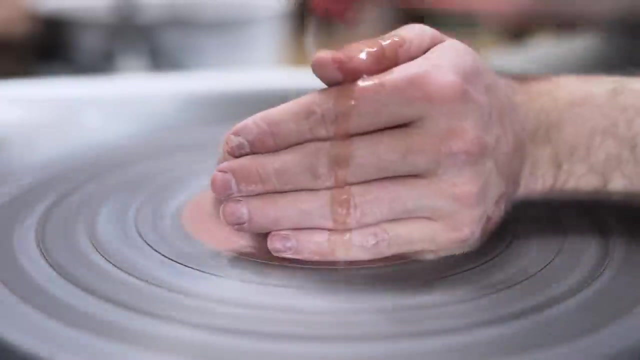 On the entire piece of clay. So don't go slowly And don't go at a medium pace. Instead, push it just that bit further. Another thing I often see beginners do Is they push this part of their hand Too firmly against the metal of the wheel. 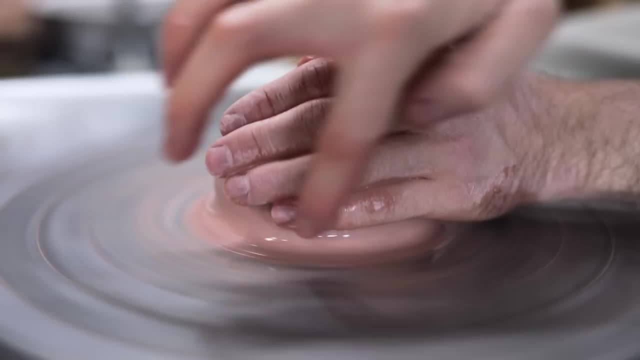 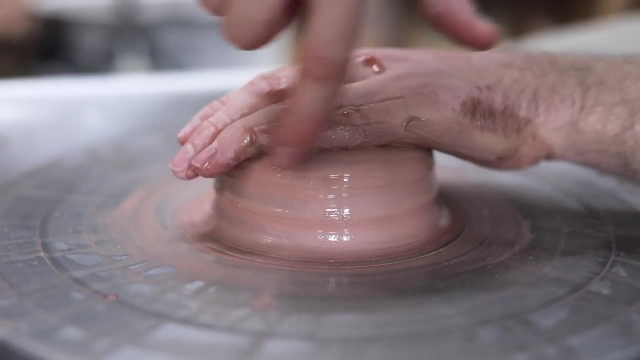 To a degree that the metal Can almost wear away the skin And become quite painful to centre. You never want to push these fingers directly down Onto the metal wheel head And you'll know if you're pushing too hard against the metal. 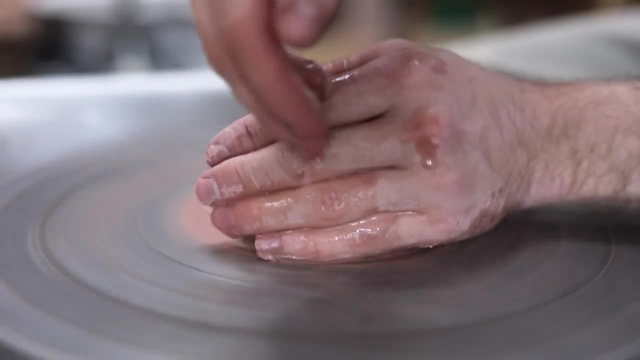 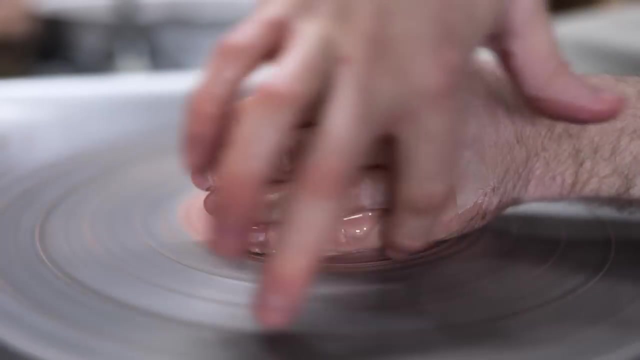 If you can see this metal residue coming off on your hand. Instead, you want to just glide Above the metal, Ideally with a thin skim of slip Between the two, Which will naturally accumulate as you centre the clay, And you'll hear when you're pushing. 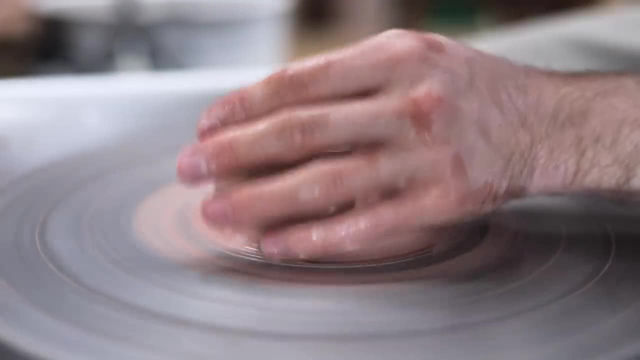 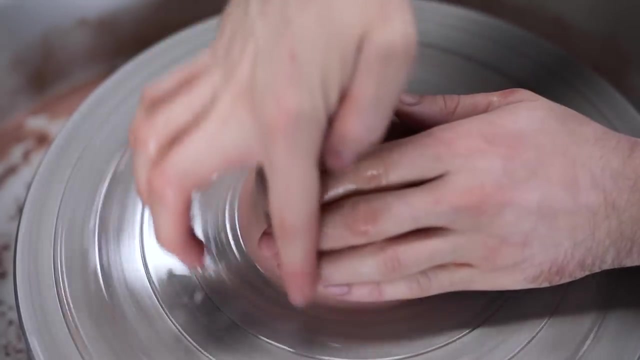 So if you feel the friction on your hand And hear the grinding noise, Just lift your hand up a millimetre or so, So it's above the spinning metal. Another thing I do to ensure that the clay is centred Is I watch my fingertips. 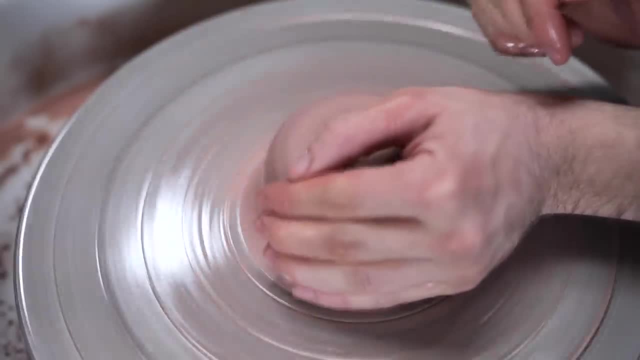 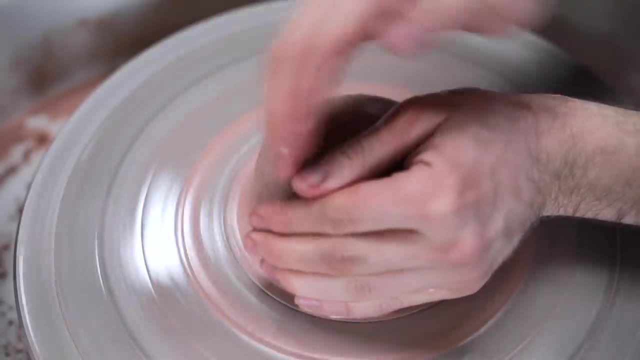 Instead of the clay itself. If the clay is off centre, My fingertips will wobble Along with the clay, And if I notice that, I squeeze my fingertips inward Against the clay And I really focus on them, not wobbling whatsoever. 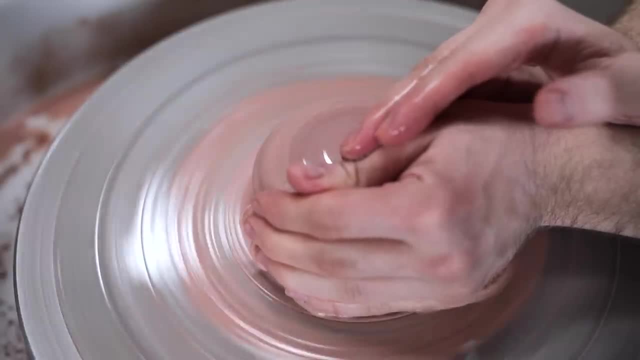 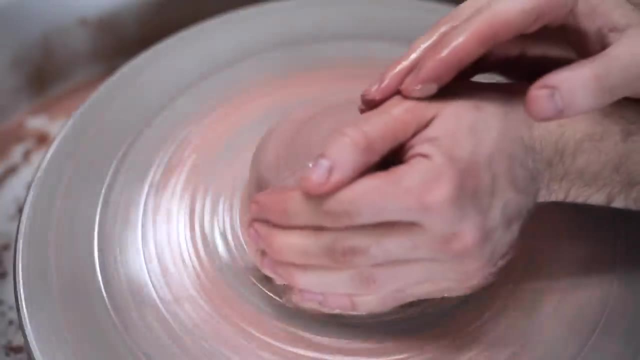 They're firmly tensed And if they're unwavering Then the clay underneath them should be quite centred. So if you watch that again, I basically knock the lump off centre. I lean the palm and the ball of my thumb. 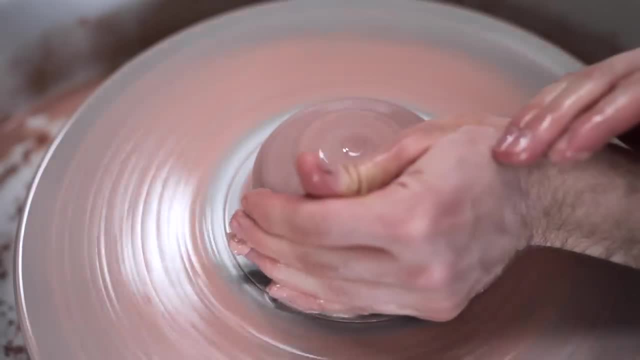 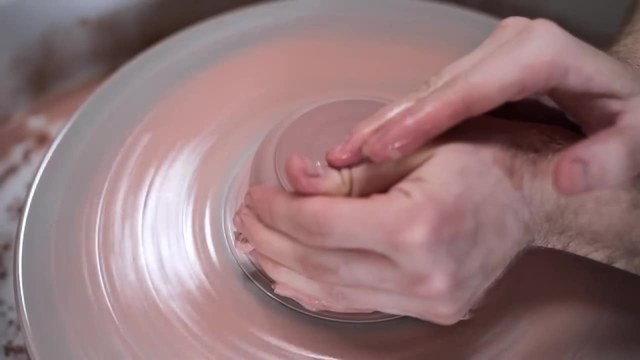 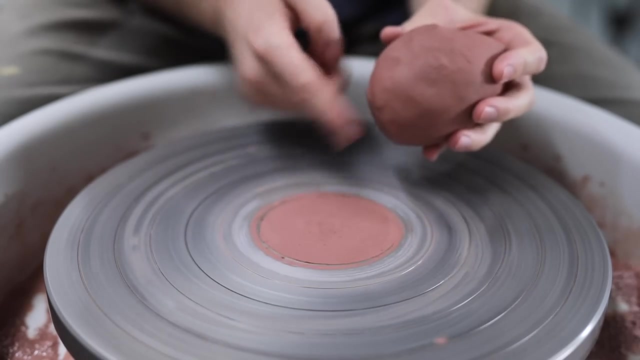 Of my left hand Into the block of clay, Pushing forwards, And then I tense those wobbling digits So they're completely still, And then I take my right hand And bring it down on top And compress, Sometimes in between pots. 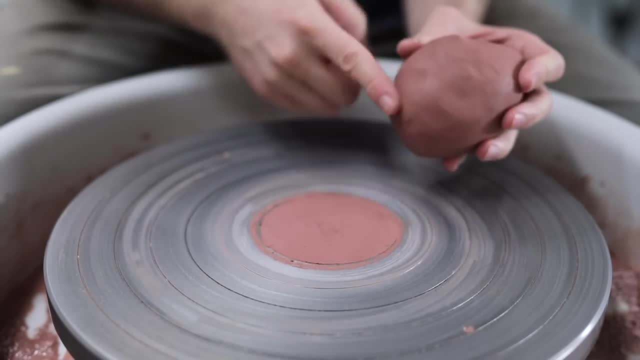 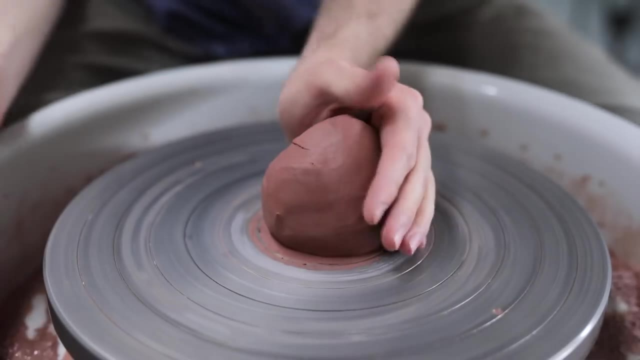 You'll have this skim of dry clay left, And I often see people remove it in between throwing new pots, Which is something you shouldn't do Otherwise. Like Velcro, Once firmly attached, I can begin to centre as normal, But this time I'm going to introduce a new element. 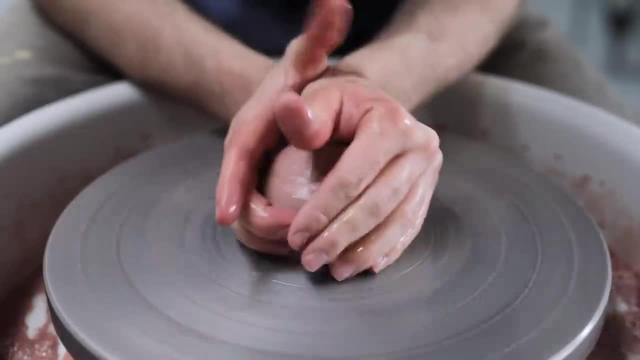 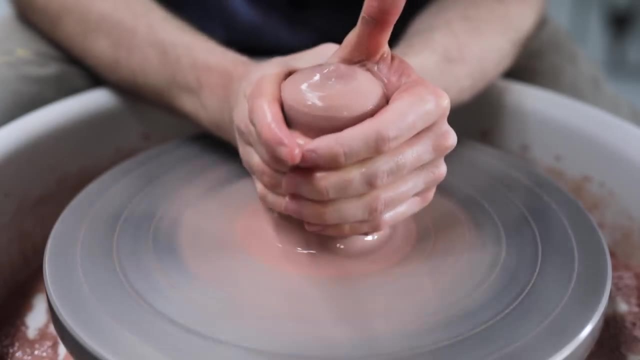 Which we call coning. This is when the lump of clay is coned Up and down Between the palms of my hands. This is almost like wedging the clay, But on the wheel, And with each cone up And each cone down. 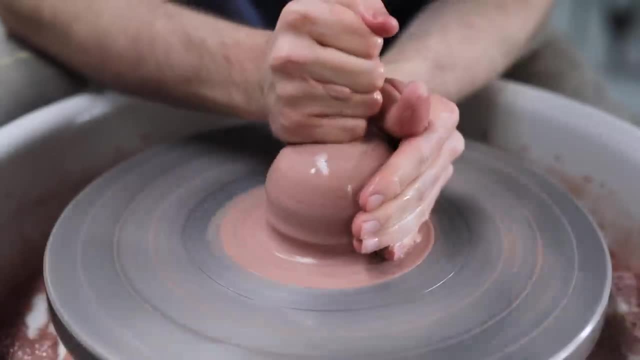 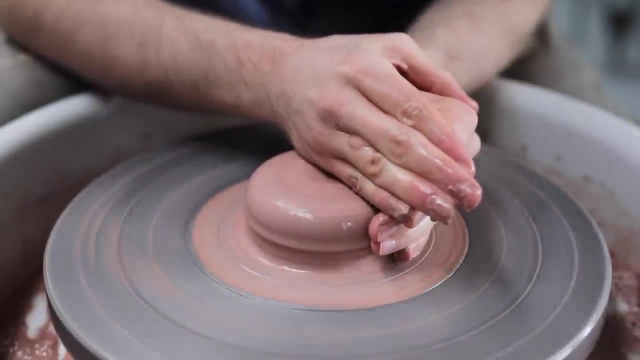 You'll feel the clay becoming more orderly beneath your hands. The analogy I use Is to think of clay like a bag of rice: Before it's been wedged. All the grains are facing in all kinds of directions. They're completely mixed. 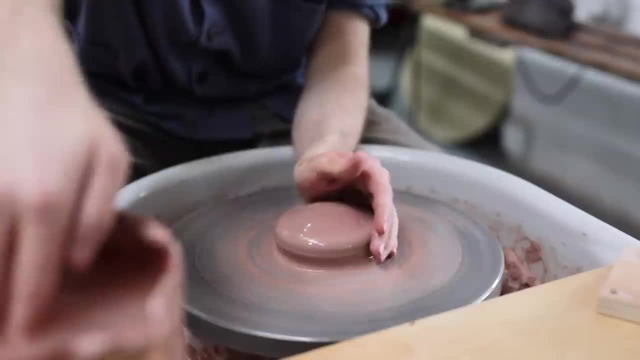 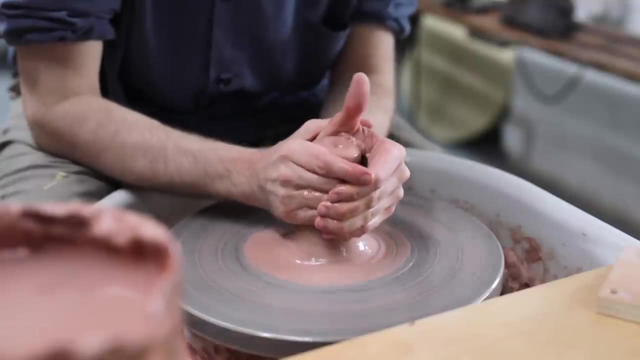 And there's no order. But as the clay is coned down, It causes the platelets to collapse onto one another And align, Facing the same direction, And in turn this makes the lump of clay more plastic And more easily throwable. 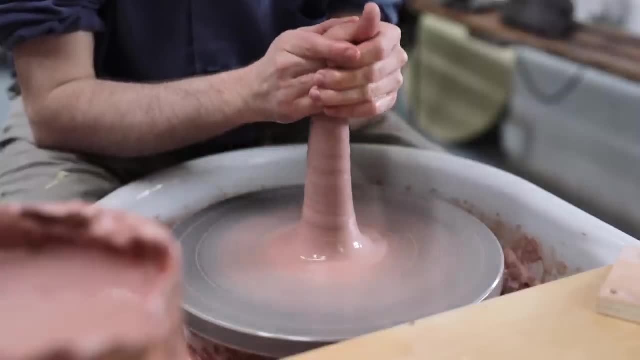 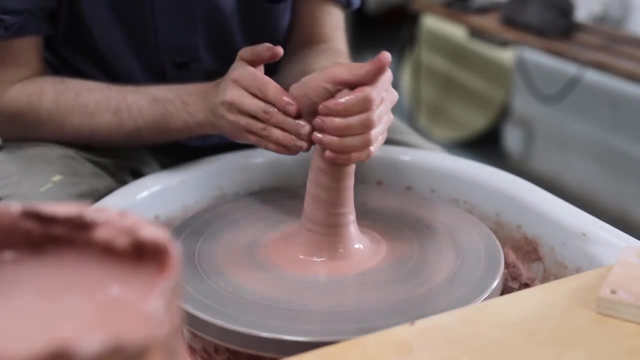 So I cone the clay up Carefully As I apply downward pressure, So I tend to push the cone both forwards And down In the same motion, And this causes the clay to bulge towards the base of the lump, Which keeps it quite manageable. 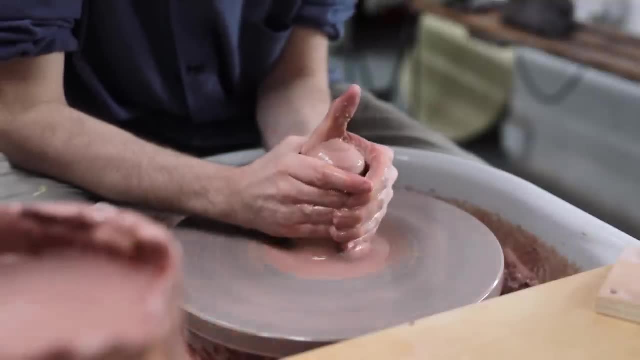 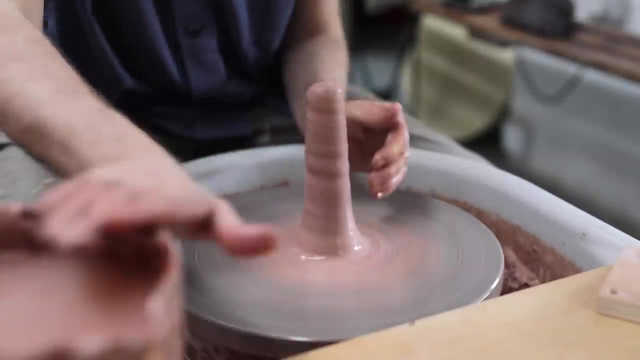 And easy to work. If, on the other hand, You cone the piece of clay up And then just push it directly down, The bulge of clay will begin to accumulate directly in your hands, Which makes this process quite difficult to control, Like you'll see here. 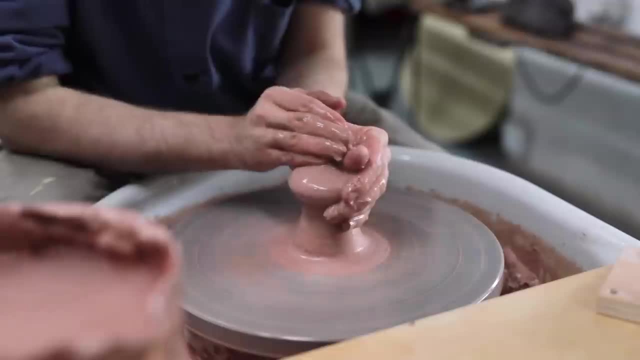 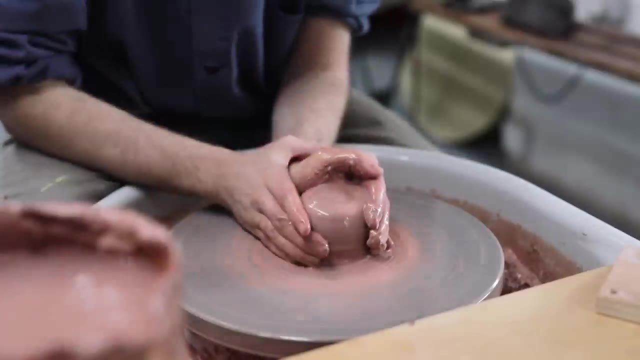 The point of coning Is that even sometimes With really thoroughly wedged clay, The lump might spin with some kind of irregularity Within it. But after you've coned it up three or four times, The lump of clay will begin to feel wonderfully smooth. 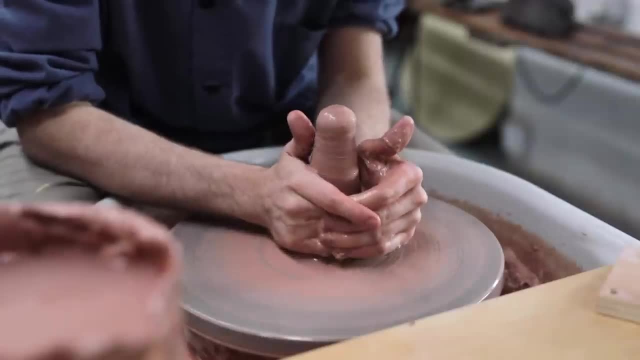 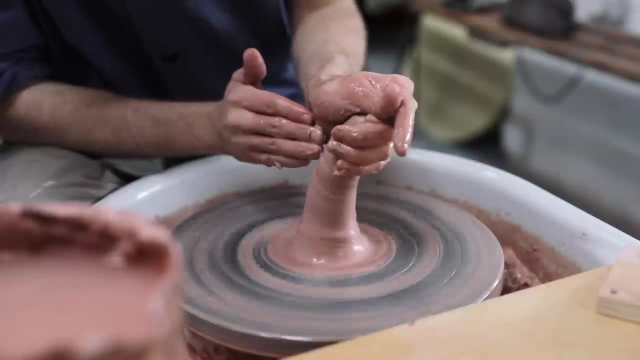 And you should have an easier time Opening up the lump And pulling up the walls of clay, Which will be the topic of my next very in depth video Like this one. So I lean the clay over to one side And, as you can see, the bulge begins to build up. 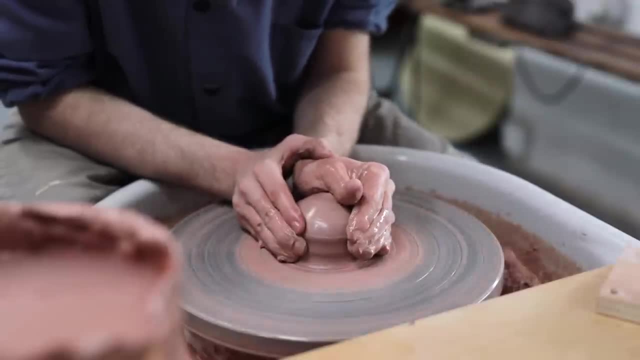 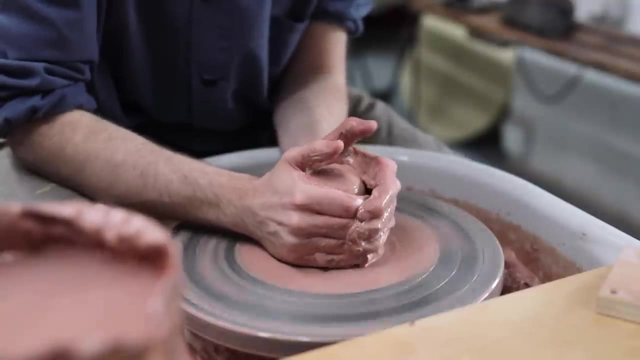 Towards the base. So that's coning And it's worth learning, And it's worth practicing And it can sometimes make all the difference, For instance when I'm throwing larger masses of clay Or pots that are perhaps a bit more complicated. 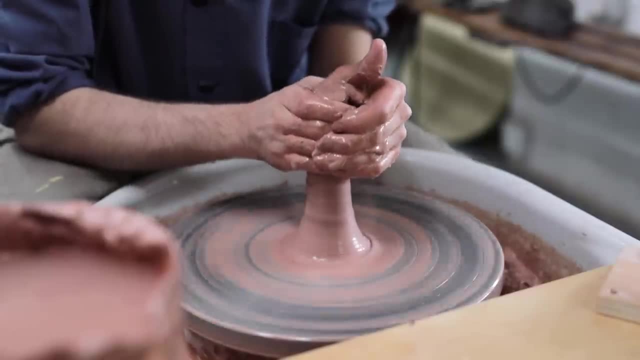 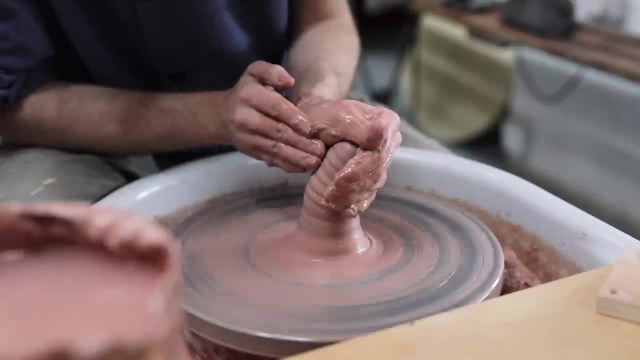 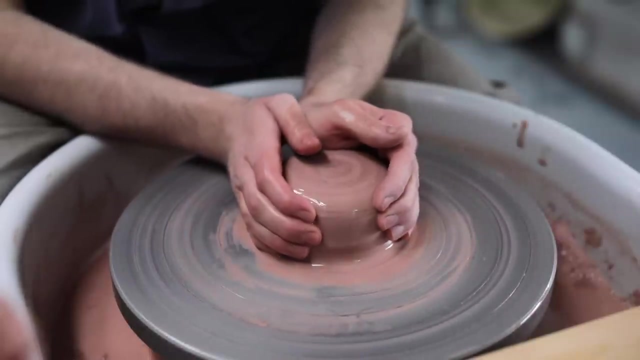 Than a mug or a bowl. I'll always make sure to cone the clay up and down A number of times. This next tip is perhaps a bit more subtle in nature, And it has to do with how you place your hands Onto the lump of clay. 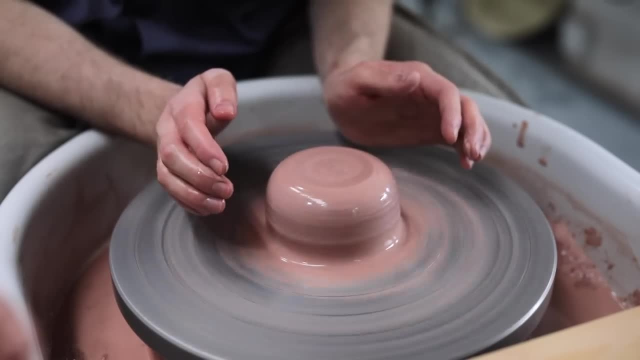 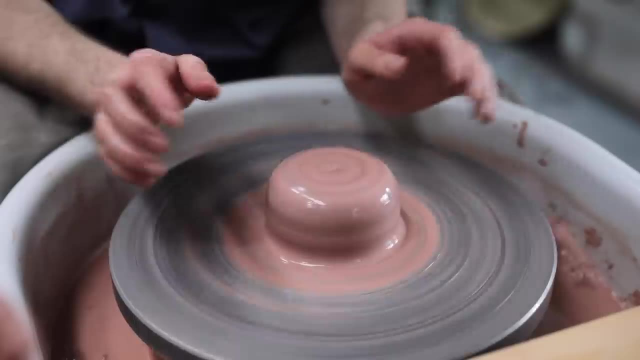 And remove them. The first thing you want to think about Is: you only ever want to make contact with the clay When it's spinning, And the same goes for when you release your hands. You never want to stop the wheel And then release your hands. 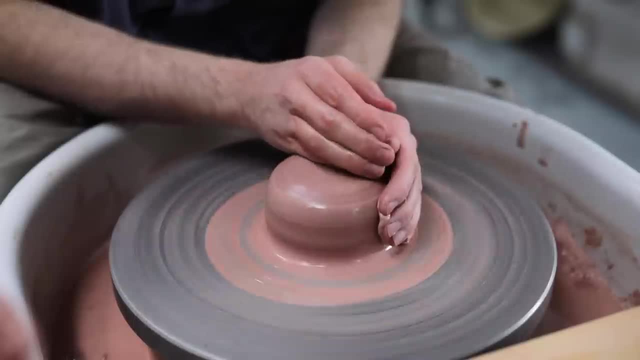 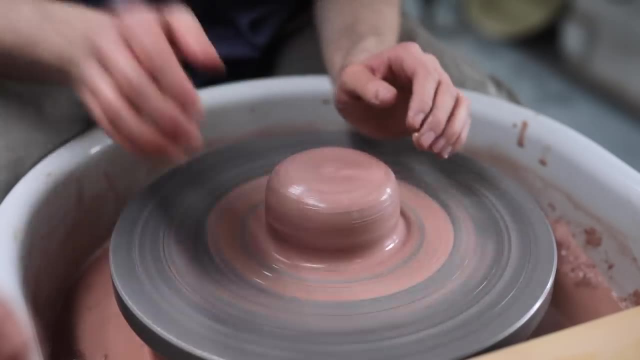 Nor do you want to place your hands onto a stationary lump And then begin spinning it. In actuality, what you want Is for the lump of clay to always be spinning When you touch it And remove your hands from it. Think of it like turning wood on a lathe. 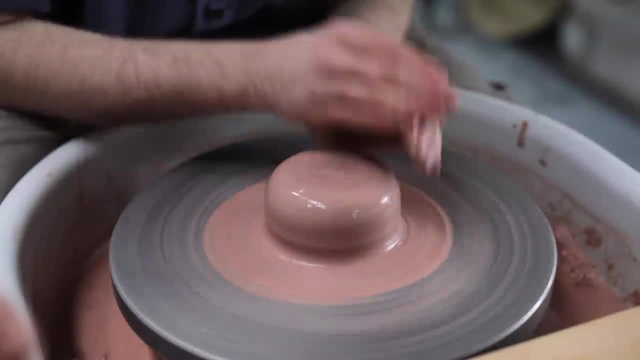 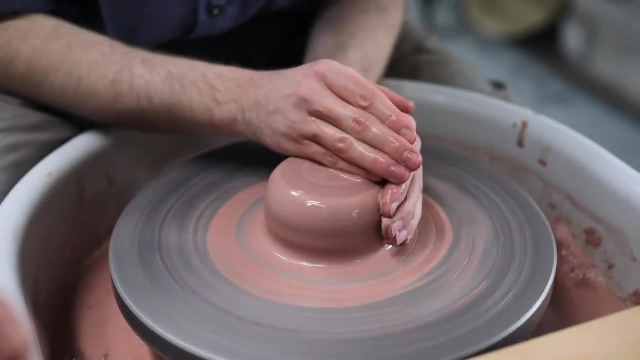 And when you're turning wood on the lathe, You always want the piece to be spinning Before you try to do anything to it, And the same goes for clay. Another thing to think about Is how you release your hands From the lump of clay. 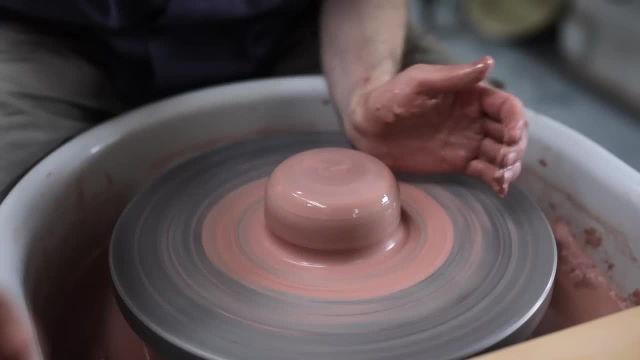 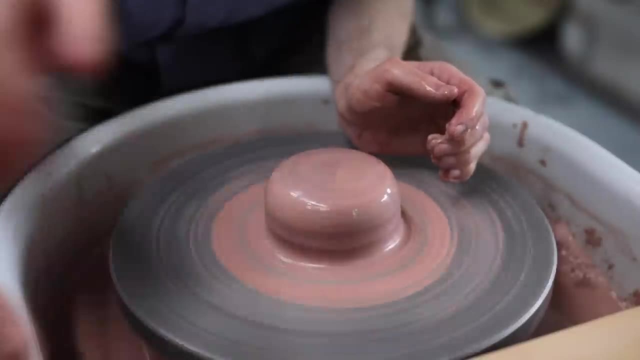 Ideally, you want to release them very gently, Like so As if you release your hands too abruptly, Like this. You'll notice, if you look carefully, A very slight wobble in the lump of clay And, if you do this, To form the base. 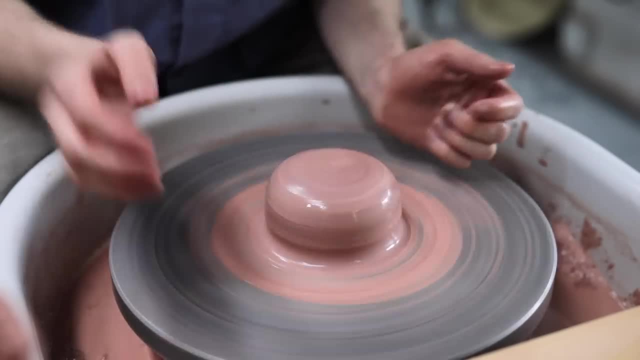 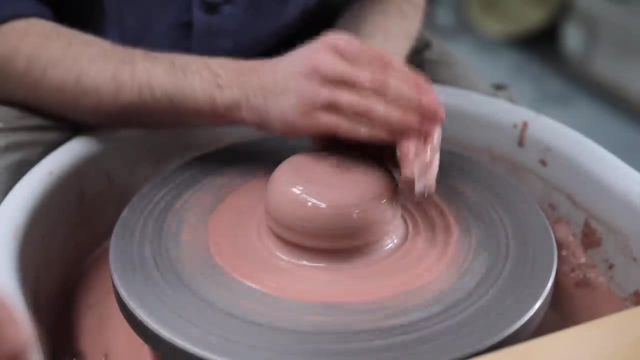 The pot could become slightly off centered, Even when you thought you centered it perfectly. Placing your hands onto the lump of clay Isn't so important, As you can immediately center them and hold them still, But when you release your hands, You want to do it very gently. 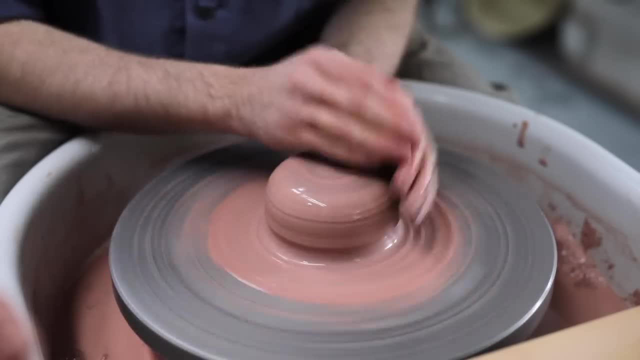 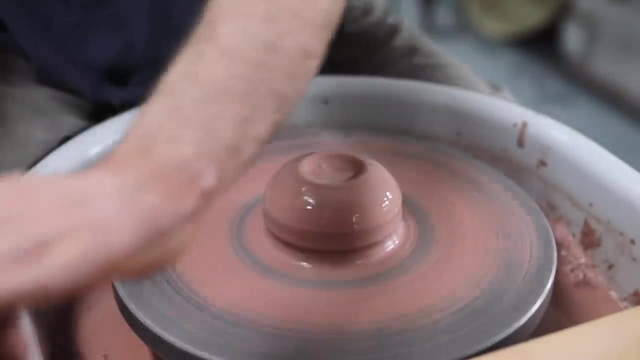 Just to detach any connection they might have. And with enough practice, It just looks like you're removing your hands normally. Being able to center well Is vital for learning to throw on the wheel. It's the first step in the process of throwing a pot. 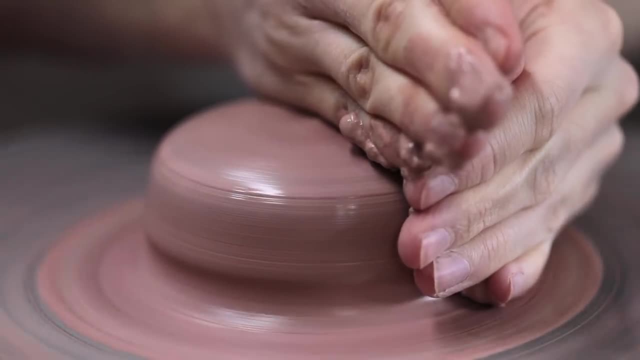 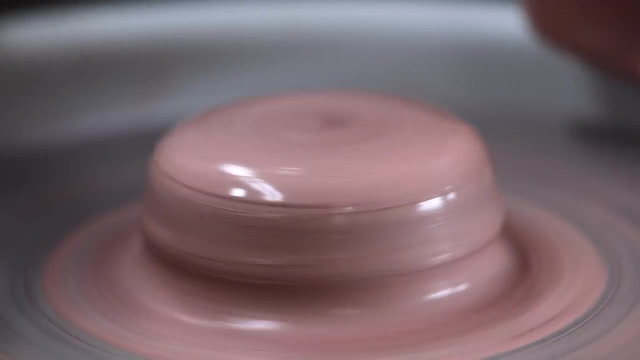 If done improperly, It makes the entire process of throwing pots more difficult And at the start, when you're learning to throw, Centering can feel really difficult. I certainly remember what it was like, But after you've thrown a hundred, A thousand,